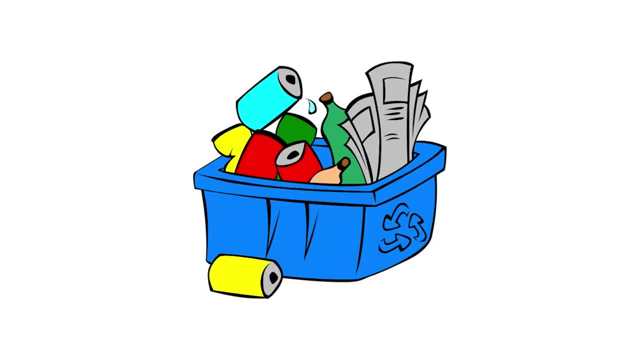 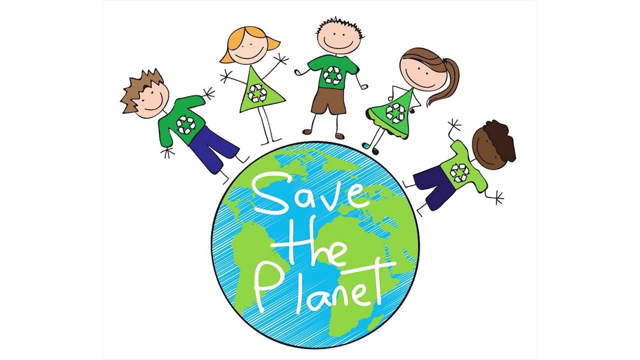 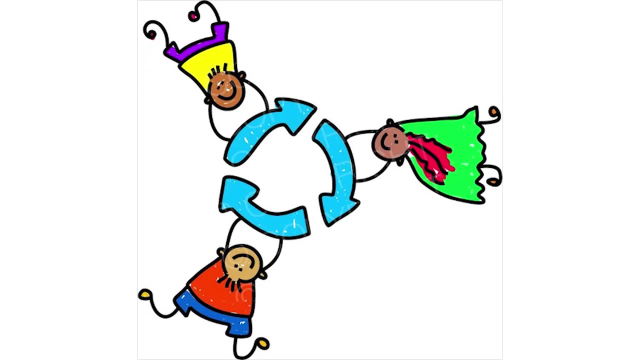 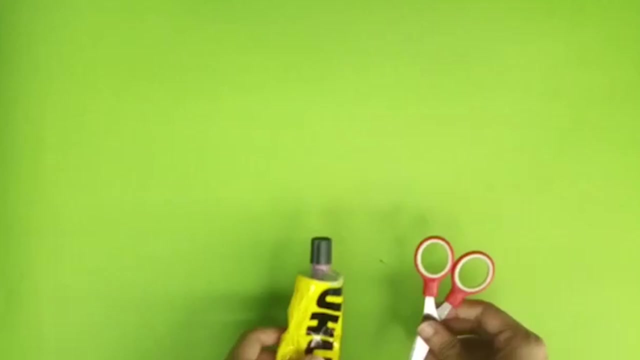 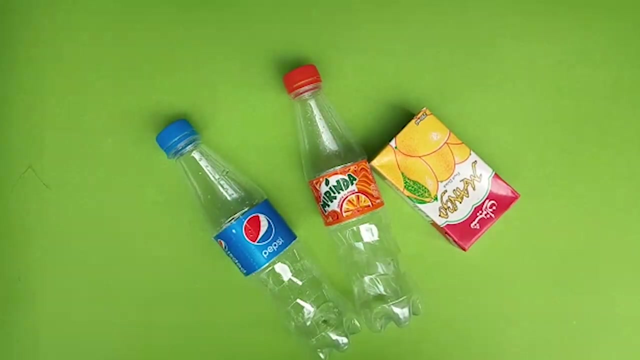 Do you know, Recycling and reusing of things instead of throwing them makes our environment clean. So in order to save our environment, we should recycle waste material. Let's make something artful with recycled material. We need some colored papers, paints and brushes, glue, scissors, some straws, plastic bottles, empty juice box crayons and some ice cream sticks. 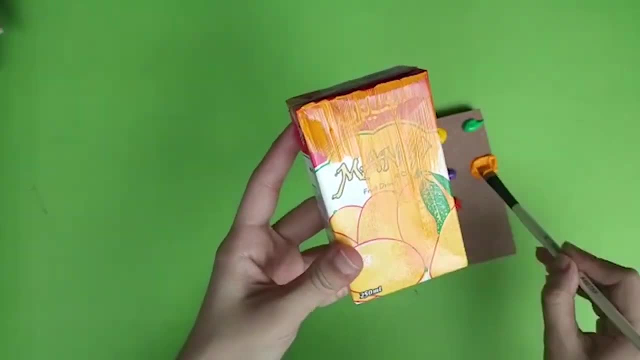 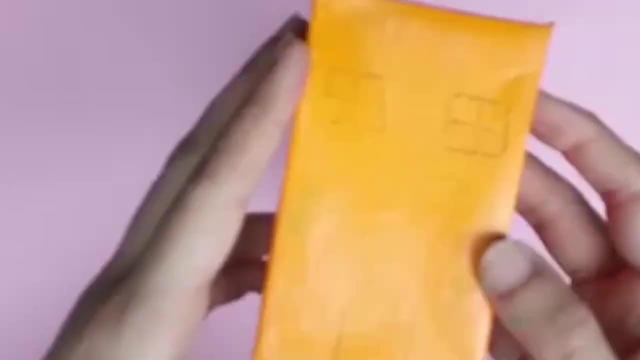 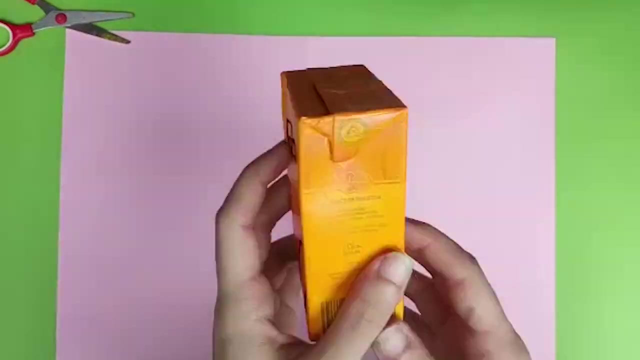 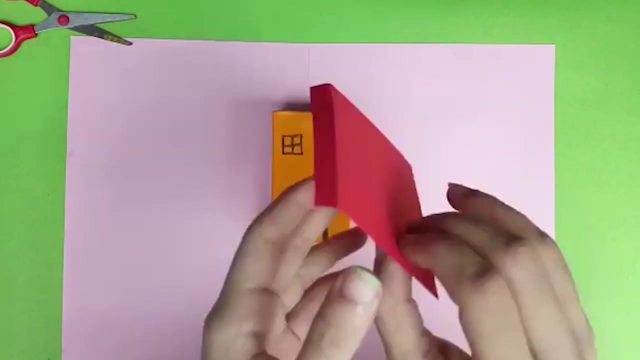 Okay, now take an empty juice box and paint it with your favorite color. Let it dry. Now draw windows and door on this colored juice box with crayons. Now take paper and paste this box in the center of the paper. Now cut a small rectangle of any colored paper and slightly fold it from its top. 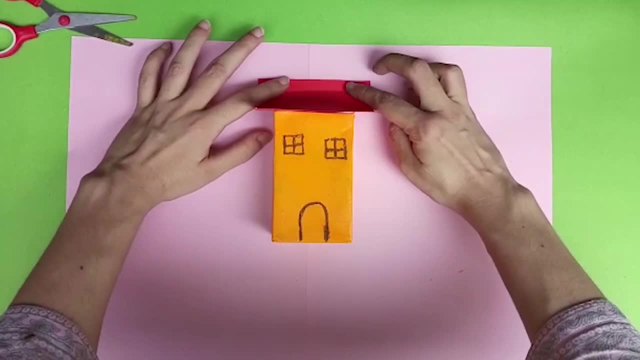 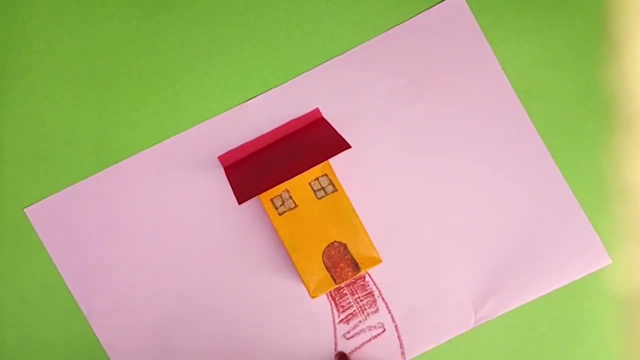 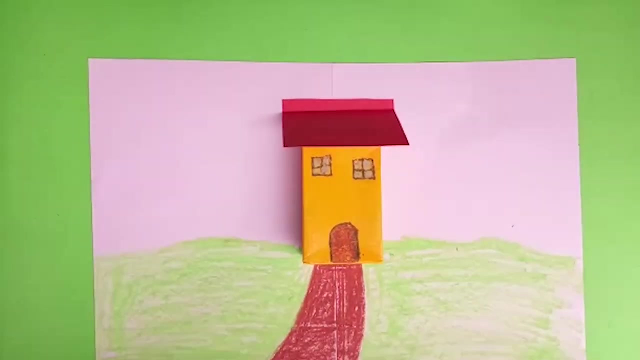 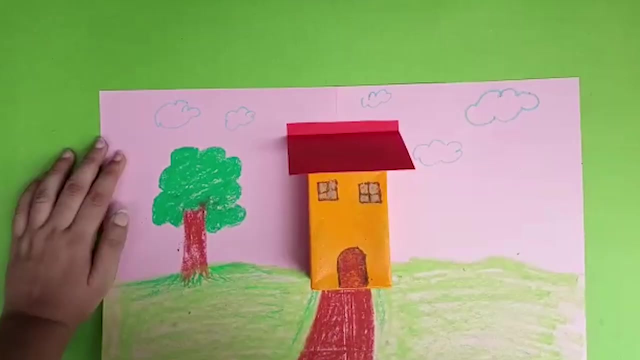 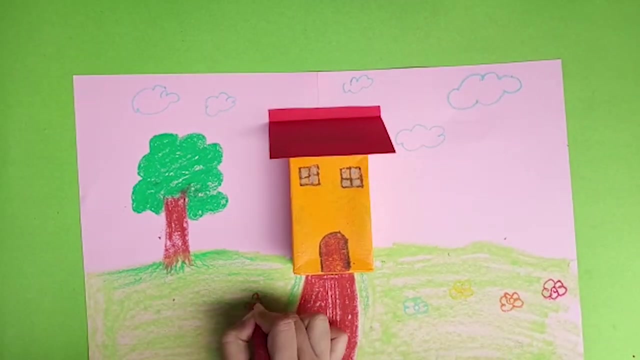 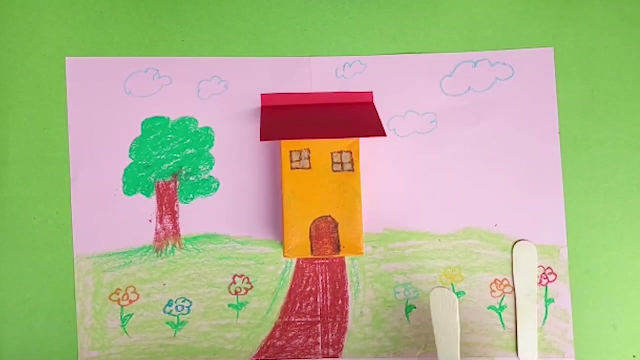 Now paste this rectangle horizontally on the top of the box. Now cut a small rectangle of any colored paper and slightly fold it from its top. Now draw grass, pathway, trees, clouds, sun and flowers with crayons For making fence. take some ice cream sticks and paste them on paper. 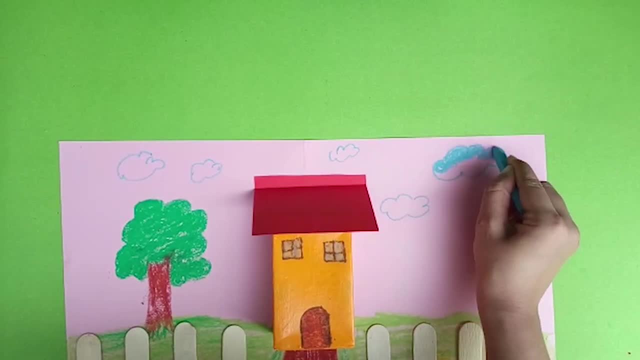 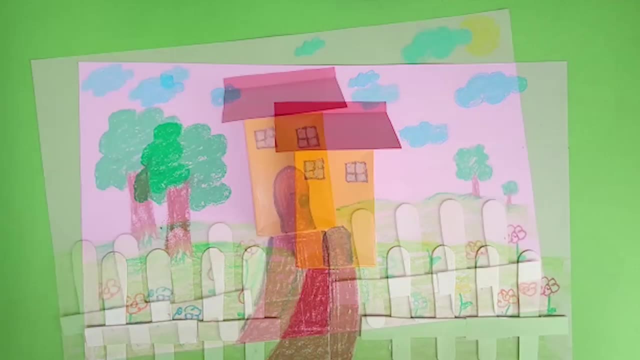 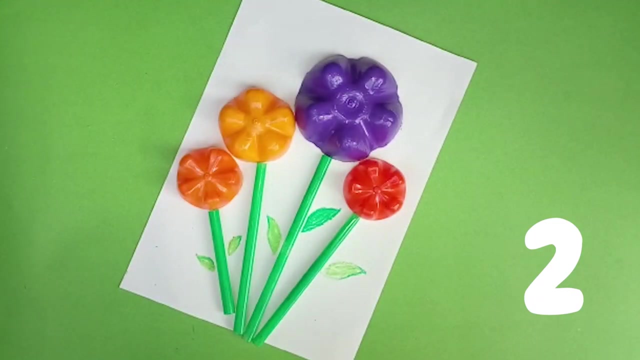 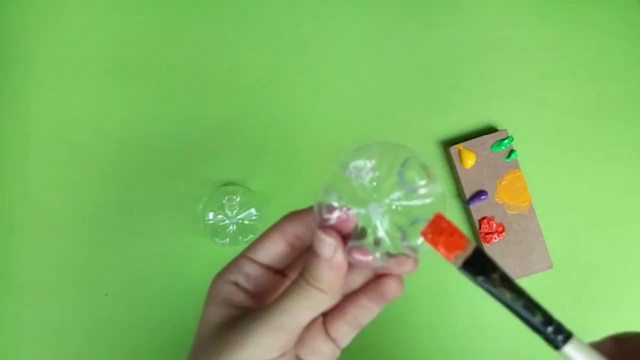 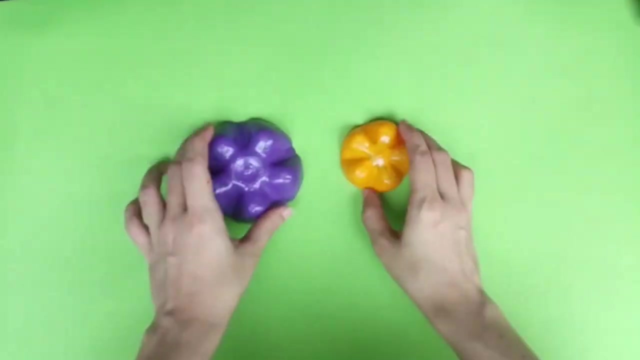 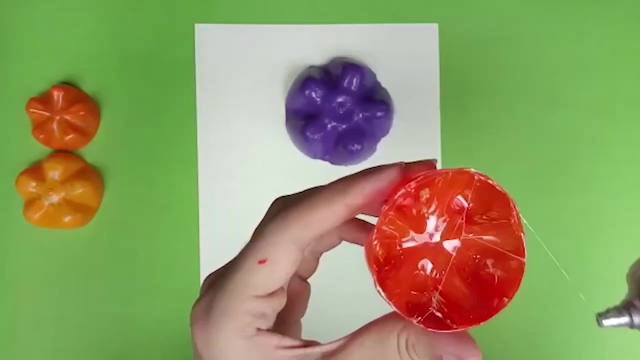 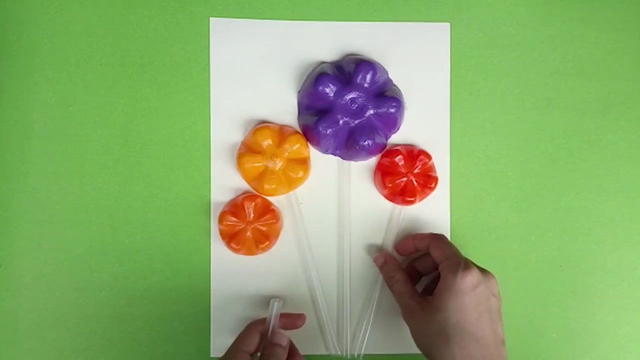 Wow, It seems wonderful. Let's try another one. Take some bottles and cut it from its bottom. Now paint these pieces with your favorite color and let them dry. Now take a paper and paste these pieces on the paper. We will use straws for making its stem.